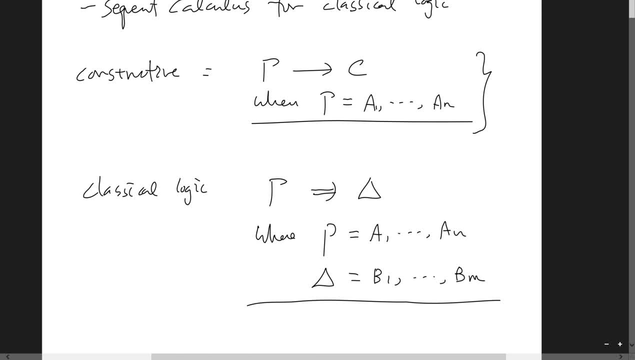 Compared with the previous form of c-quantum. here we see that the left-hand side is the same- It's just a bunch of formulas- But the right-hand side is different. In the case of constructive logic the right-hand side is a single formula, But in the case of classical logic, 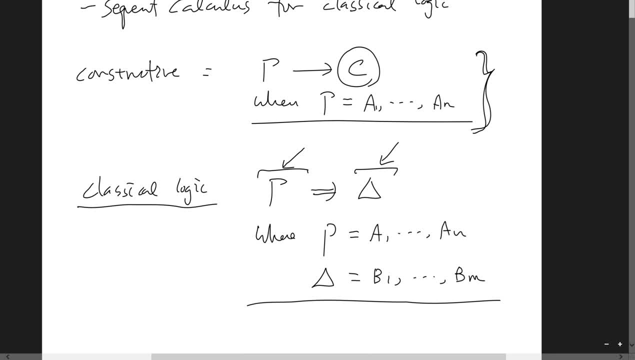 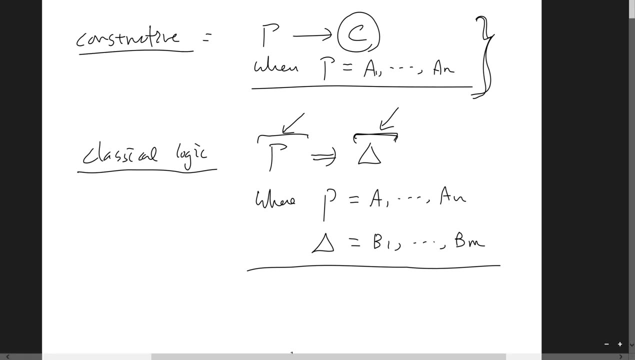 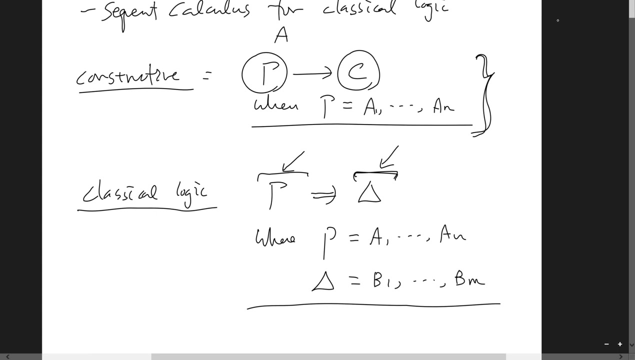 the right-hand side is a collection of formulas, So we allow multiple formulas in the right side And the interpretation is also very different. In the case of constructive logic, the interpretation was: gamma is a collection of neutral judgments. So we have, in the case of this, 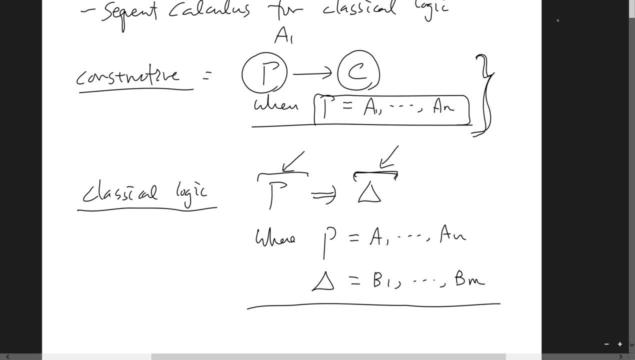 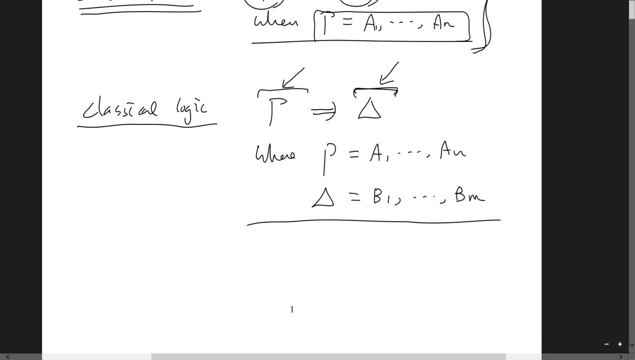 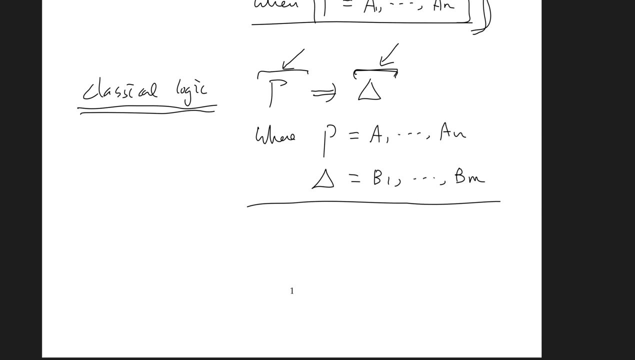 so in this case gamma is interpreted as a1 down arrow through a n down arrow, and c is interpreted as c up arrow. This is the constructive logic. But in the case of classical logic the interpretation is based on proof by contradiction. So for every formula in 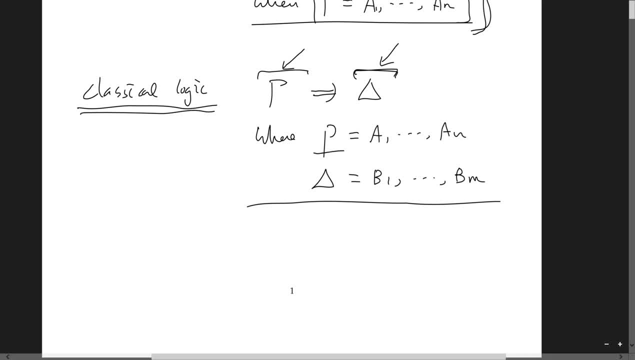 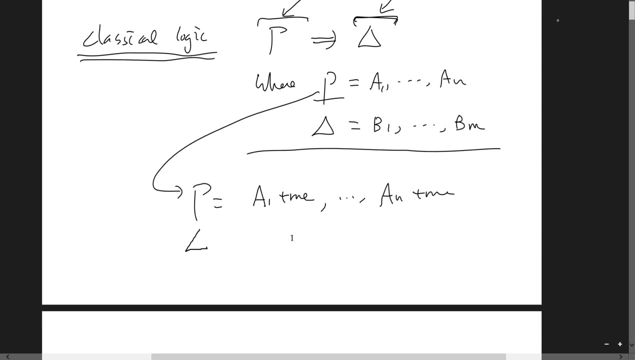 Gamma, we make an assumption of truth judgment. So Gamma is interpreted as assumption of a1 true, a1 true through An true, And for Delta, we make assumptions of b1 false through bn false. So that's the difference, That's the main difference. For Gamma, we make assumptions of truth. 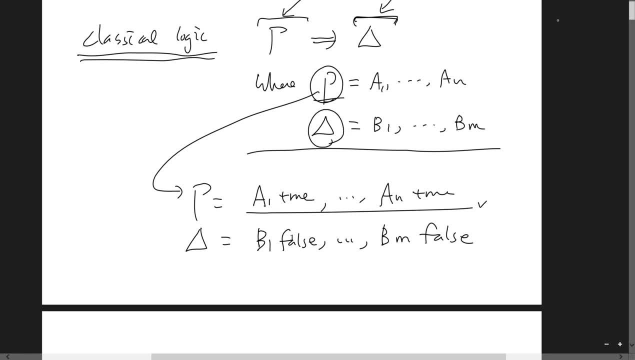 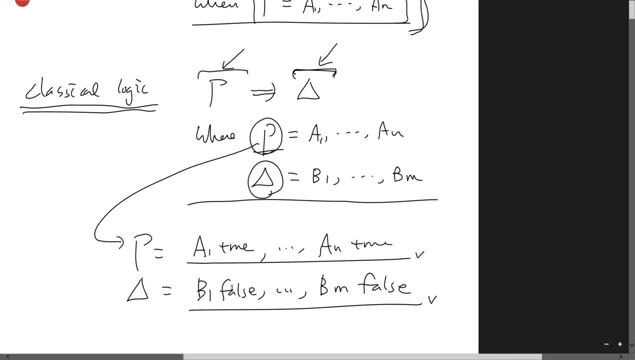 judgment And for delta we make assumptions of force of judgment. And this sequence gamma, double error. delta means from these assumptions we can produce logical contradiction. So that's the interpretation. That's the interpretation of this sequence for classical logic. The left-hand side is a collection of truth judgments, assumptions of truth judgments. 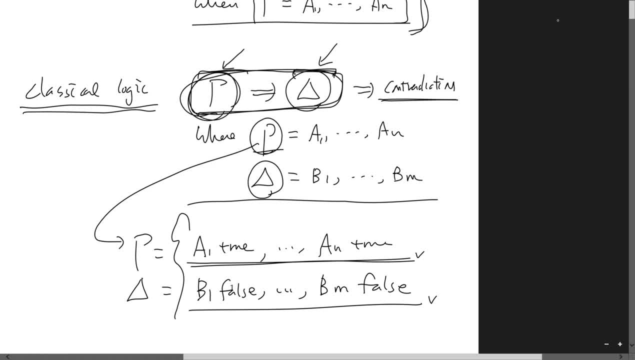 And the right-hand side is basically assumptions of force of the judgments. And from these truth assumptions and forced assumptions we can produce a logical contradiction. That's the interpretation of this sequence. So with this interpretation of sequence, for classical logic, let's develop the inference rules. 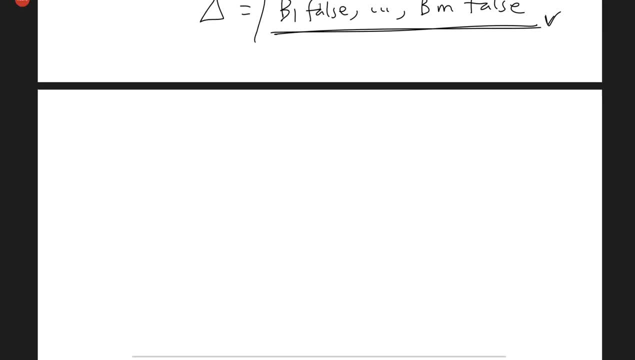 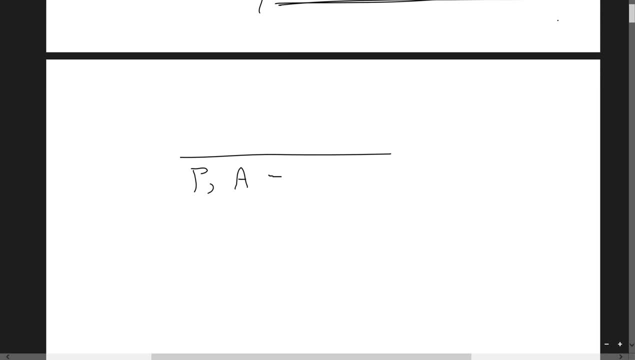 So the first inference rule is this contradiction rule. So gamma, A right arrow, A delta, And we call this rule contradiction. We call this rule contradiction rule. And it's very easy to justify this contradiction rule because, according to the interpretation, according to the definition of this sequence, this thing means we have an assumption of A true 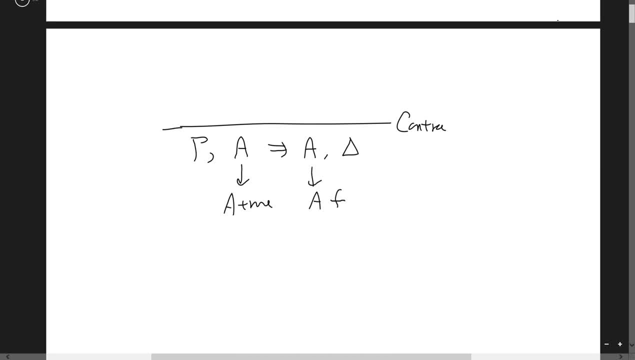 And this thing means we have an assumption of A false. So combined together these two guys directly produce logical contradiction. So the proof is complete. We have generated a contradiction from these assumptions. So this is the contradiction rule. We can compare this contradiction rule to init rule in constructive logic. 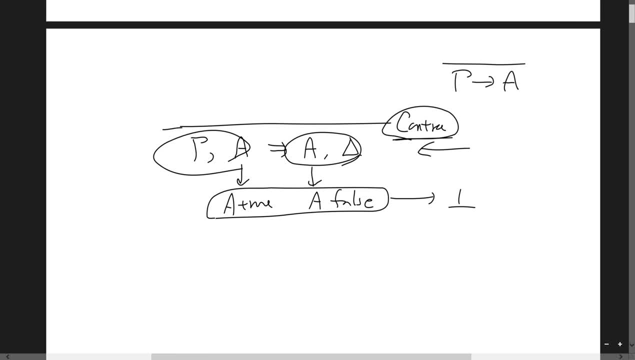 So gamma right arrow A, Oh sorry, Gamma A right arrow A, And this is init rule And in our interpretation of sequence, this thing means A down arrow And this thing means A up arrow. So we complete this hourglass where this A down arrow is converted to A up arrow. 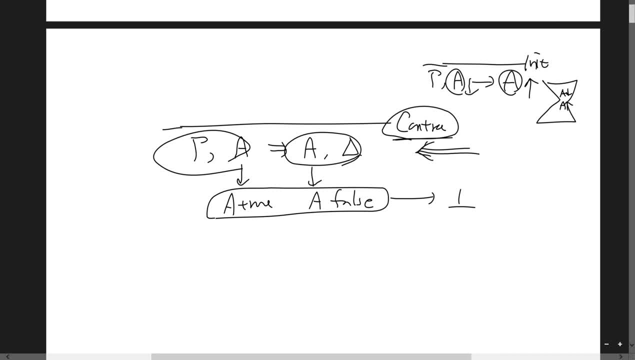 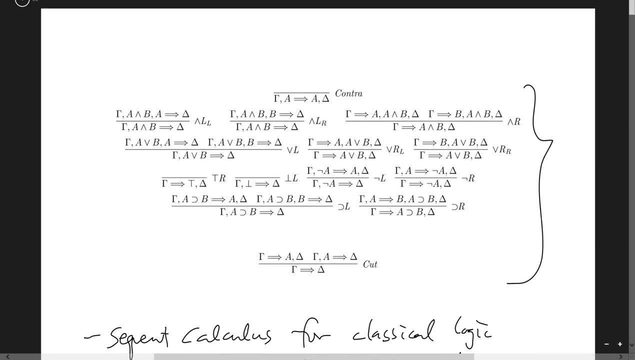 But interpretation is totally different here. It just says that an assumption of A true and assumption of A false, they lead to logical contradiction, That's all. So this is the first inference rule in the sequence calculus. So we have found this rule, contradiction rule. 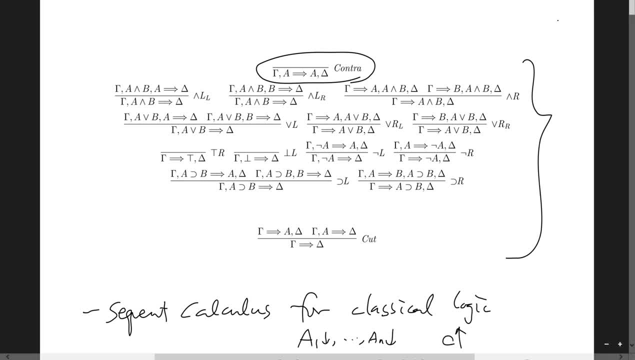 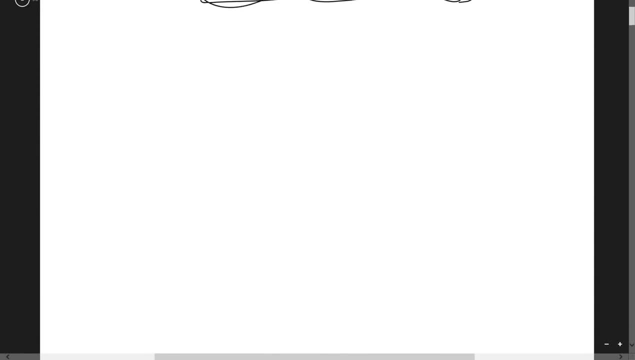 And for every logical connective, we have left rule and right rule. Let's consider the conjunction case first. Uh, If this conjunction appears in the left-hand side, this thing means? according to our definition of this sequence, it means A conjunction B- true. 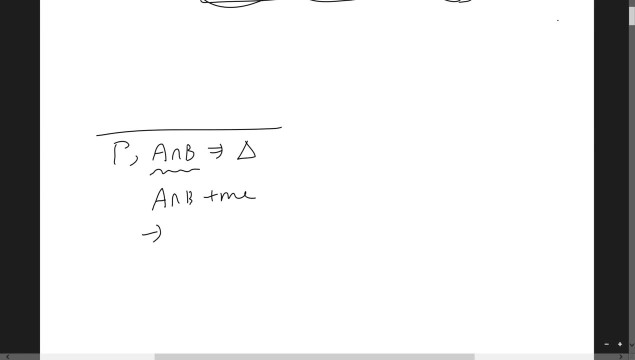 And if A conjunction B is true, we can of course deduce A is also true. That's the meaning of a conjunction. So therefore we can introduce an additional assumption of A true. So we move upward and introduce A true as new assumption. 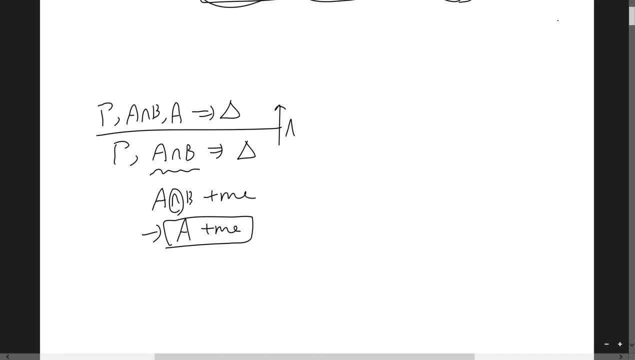 So this is conjunction left rule And we focus on the left formula here. So it's conjunction left- left And there's a symmetric case- Conjunction left rule, But this time we focus on the right formula. This is conjunction left rule, right. 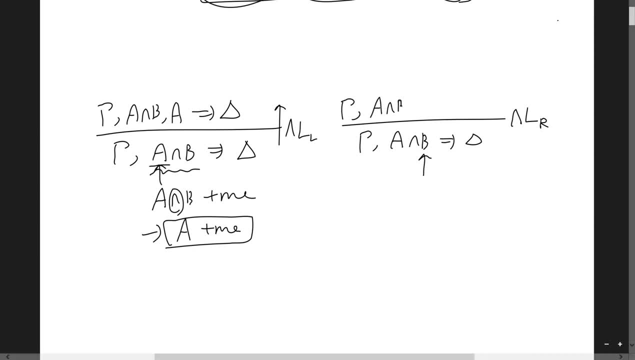 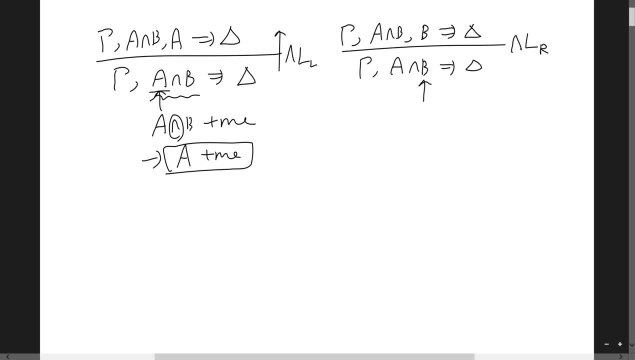 So we have gamma A conjunction B B right arrow delta. What about conjunction right rule? Gamma right arrow A conjunction B delta. This time, according to our definition of a sequence, this is interpreted as A conjunction B false. 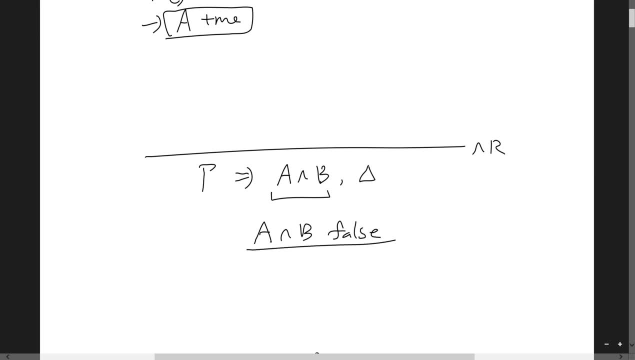 And if you think about the meaning of A conjunction, B, false, it means that either A is false or B is false. Now, from these assumptions, we'd like to create a line, A logical contradiction, And there are two possibilities. The first: A is false. 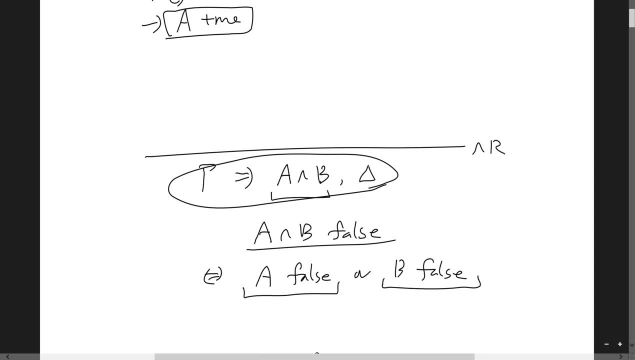 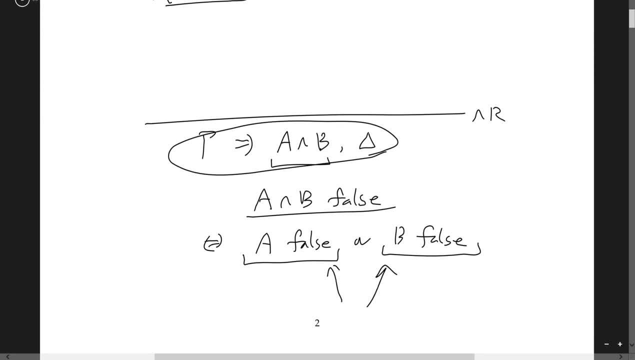 And the second B is false. So, in order to produce logical contradiction, we have to deal with both cases. In other words, we have to generate a logical contradiction from this case and also from this case. So therefore, now the premise contains: 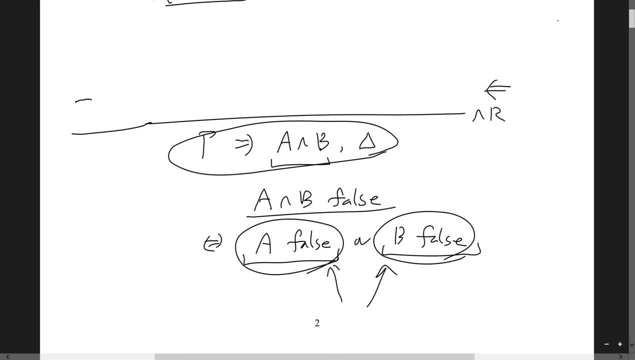 two new sequences. In the first case we take this branch, So now we have an additional assumption of A- false, So A false A, conjunction B and delta. There's no reason to remove this one, because an existing assumption can be preserved. 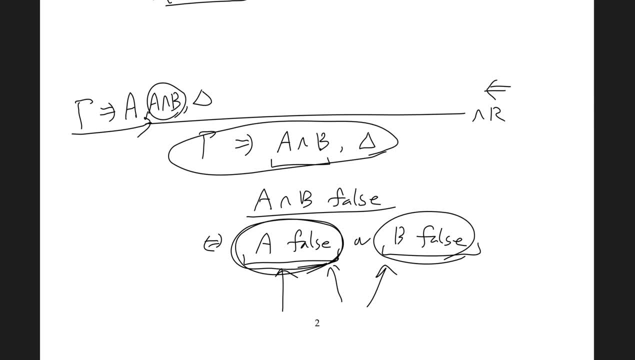 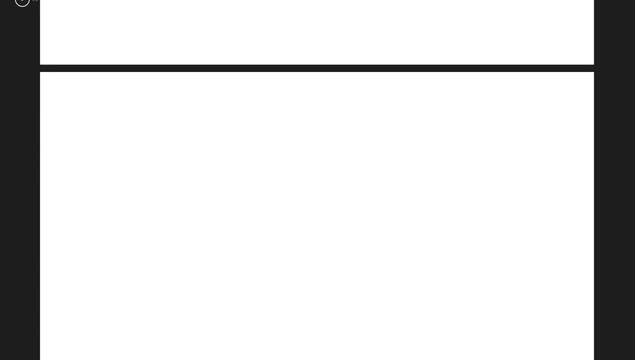 And the other sequence in the premise takes this branch, So we introduce this assumption. B is false. So gamma B A conjunction B delta, That's a conjunction right row. Now let's consider the disjunction Gamma A- disjunction B delta. 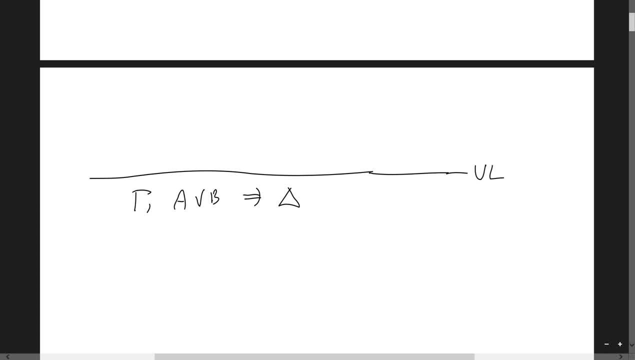 So this is going to be the disjunction left row. So we have to produce logical contradiction from these assumptions And if we focus on this one, A disjunction, B true means either A is true or B is true. So there are two possibilities. 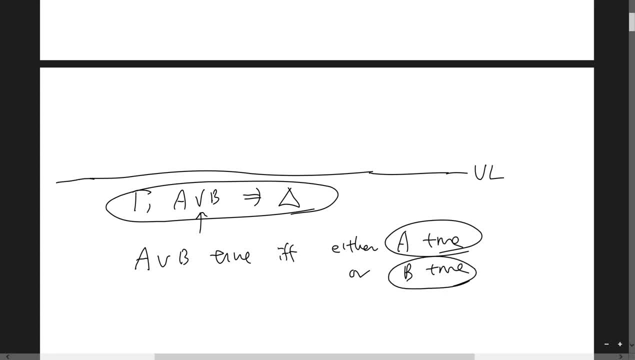 A is true or B is true. So in order to produce logical contradiction, we have to consider two cases. The first case, A, is true, And the second case, B, is true. In the first case, we assume A is true. 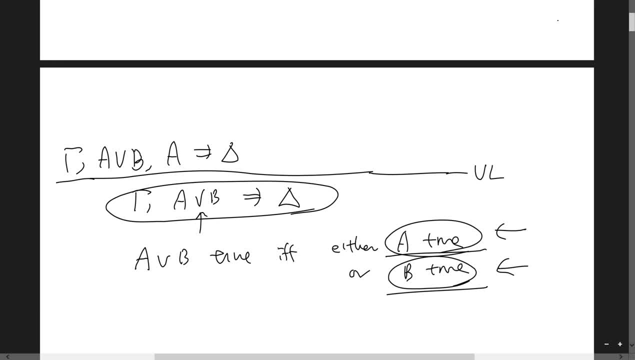 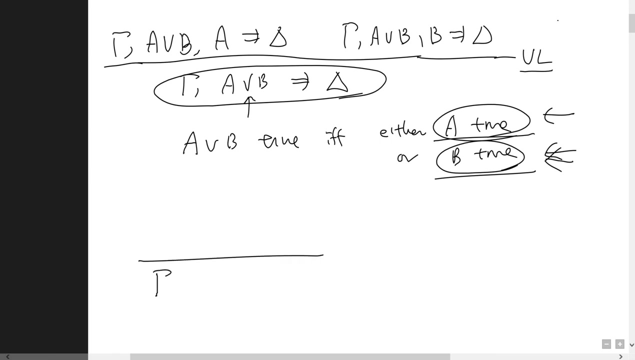 So we have this sequence And in the second case we assume B is true And then we generate the logical contradiction. So this is a logical disjunction left row. What about disjunction right row? Suppose that we have A disjunction B delta. 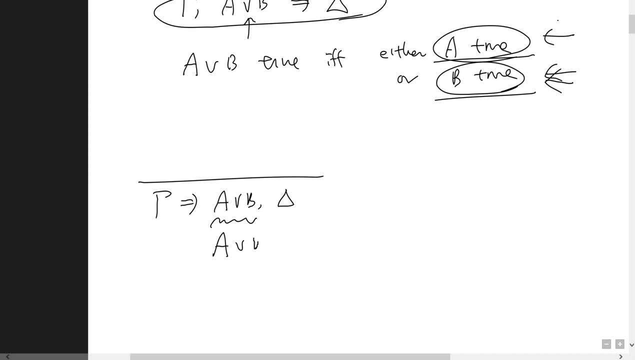 So this is interpreted as A disjunction B false. A disjunction B false is A or B is false And if we think about the meaning of A or B is false, we can show that A must be false. Otherwise, if A is true, 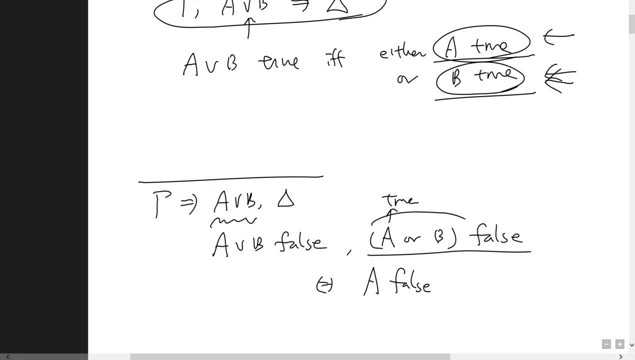 then the whole formula is already true. So that can't be the case. So therefore A must be false And also B must be false for the same reason. So if we have an assumption of A disjunction B false, we can safely assume that. 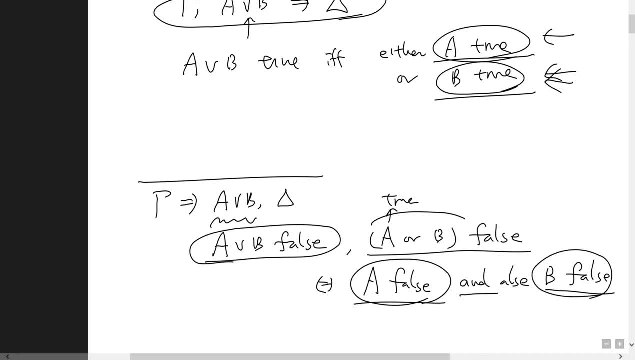 A is false and also B is false. So if we move upward, we can introduce an additional assumption of A false, which is justified by this: A disjunction, B false, And this is a disjunction right row, left And there is a symmetric case. 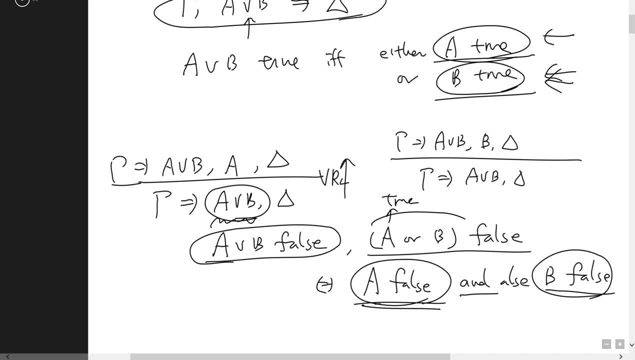 A disjunction B, B, delta. So this is disjunction right, row right. So notice that we don't discard A disjunction B here, And in fact we should not discard because we may actually focus on this formula again in order to produce. 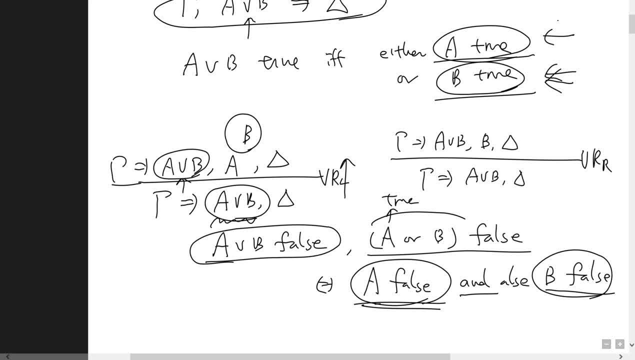 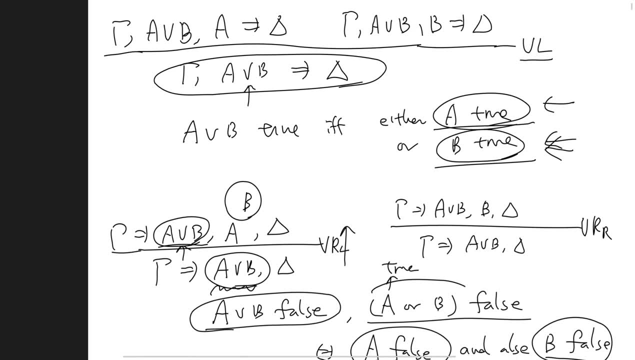 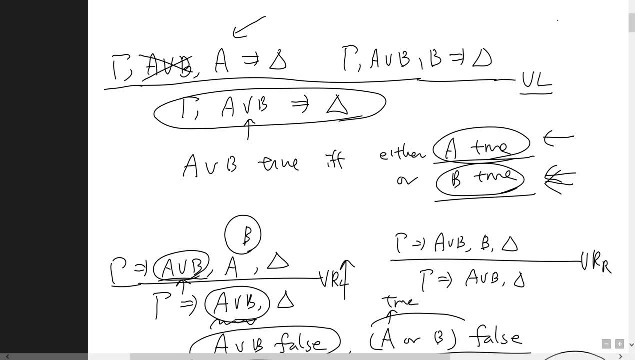 an extra assumption of A false, So you don't want to get rid of this. However, in this case, in practice, you don't actually need this A disjunction B here, because we have a stronger formula: A true. A true always implies: 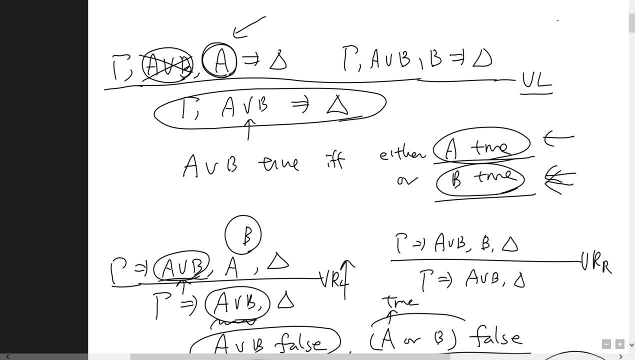 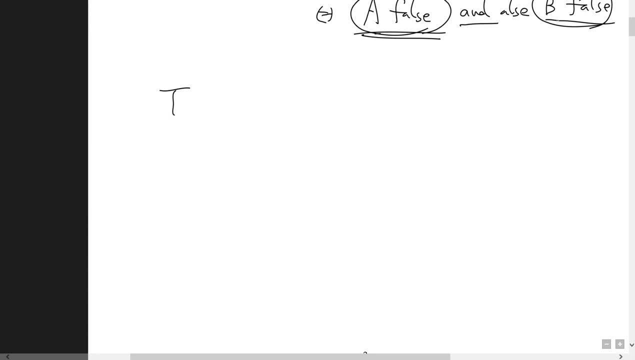 A. disjunction B: true, So it's okay to remove this formula, But for consistency we leave this formula in the premise. Now let's consider this top and bottom. If top appears on the left side, there's nothing we can do. 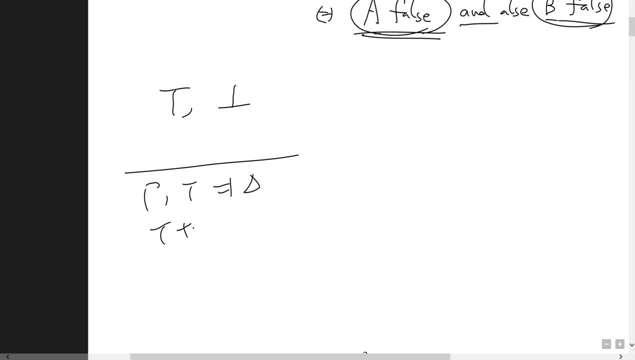 about it because top true is always guaranteed, So there's nothing we can do about this top, the formula top appearing in the left side. So there's no rule. So what about top right rule? So, according to our definition of this sequence, 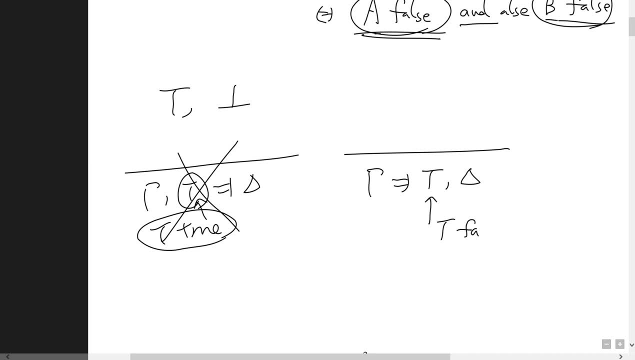 this thing means top is a false. But top by definition. top can't be false because by definition it is true. So we have already generated the logical contradiction. The presence of top in the left side automatically implies a logical contradiction. So the proof is complete. 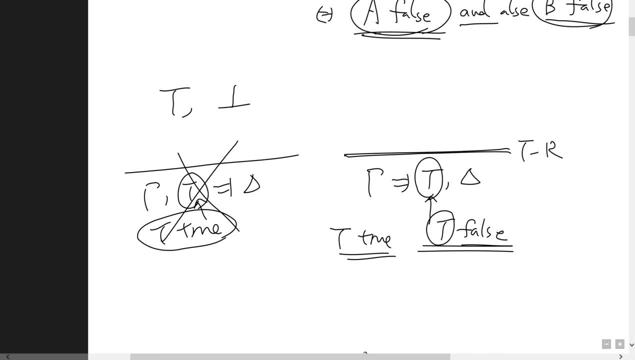 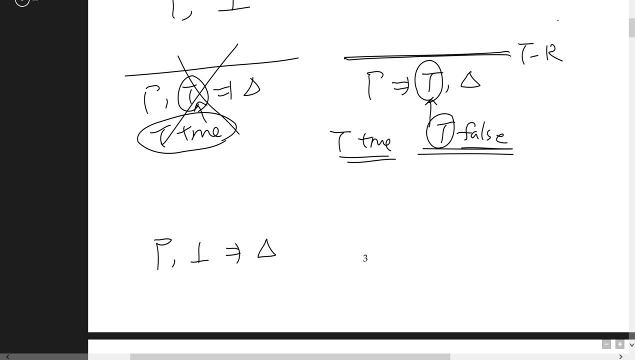 So this is top right rule. What about bottom? Similarly, if bottom appears on the left side, we have: bottom is true. So we have already generated this logical contradiction, So the proof can be completed. So, top, sorry, bottom left rule. 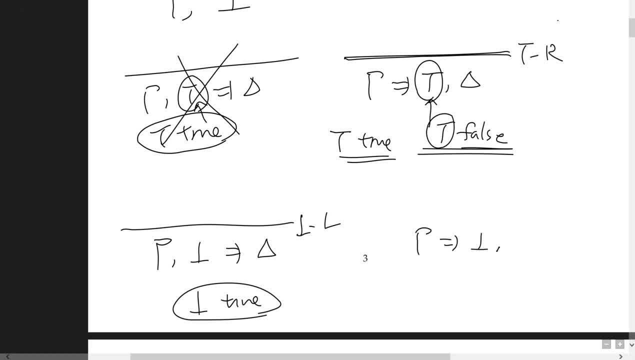 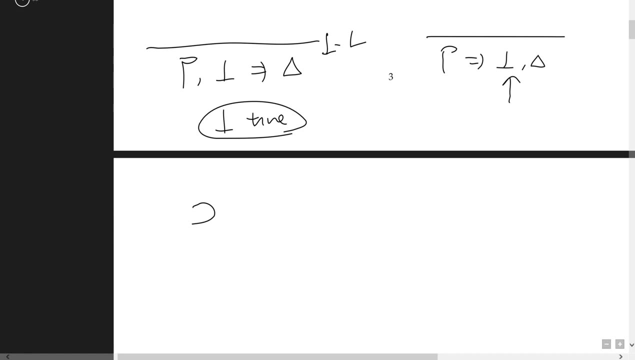 And similarly there's no rule for bottom right because there's nothing we can do about it. So finally, we need these inference rules for implication. But it turns out that in classical logic we already have conjunction, disjunction and top and bottom. 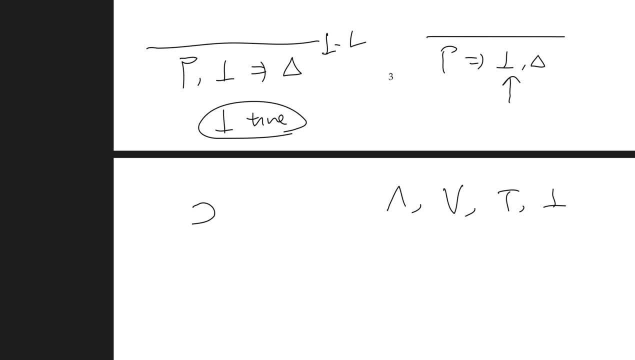 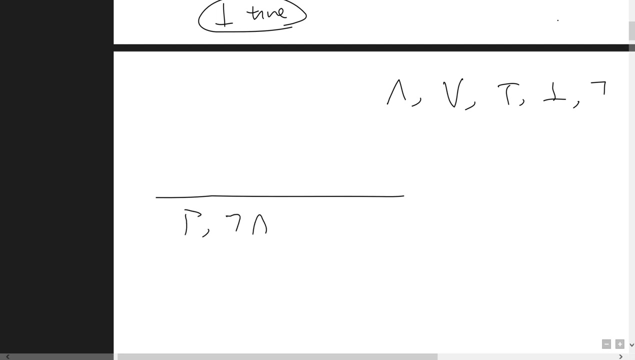 And it turns out that we don't need this implication. But let's first consider. I missed this negation, So let's consider negation. So what happens if negation appears on the left side? Well, negation A true means that our interpretation of 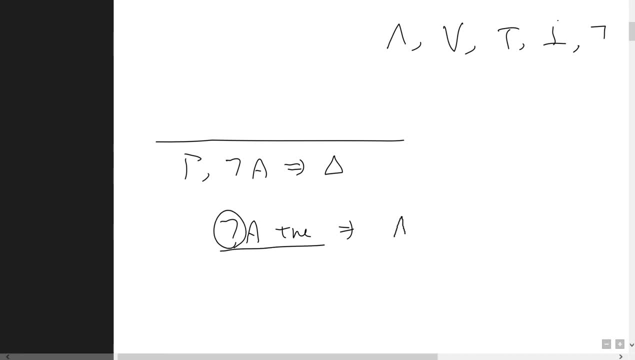 negation is well, negation A true means A is false. That's how we internalize the knowledge of A being false using this negation, the logical connective negation. So if we move upward we can generate a new assumption. 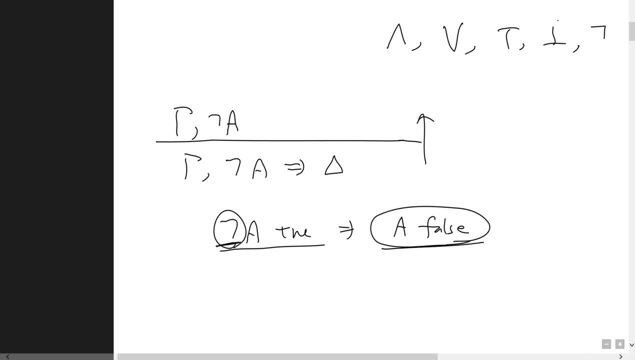 A is false, So we move upward and we assume A is false, So A is false And we try to generate logical contradiction Again. notice that we don't actually get rid of this negation A It's okay to get rid of. 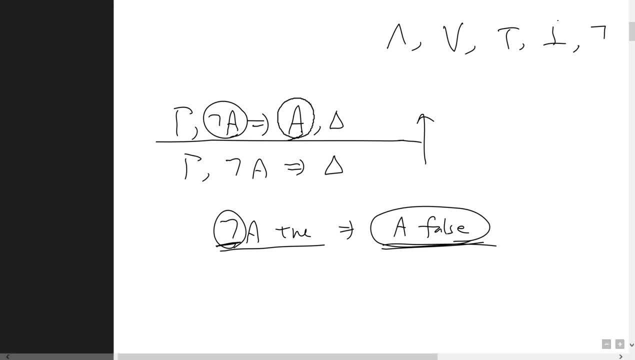 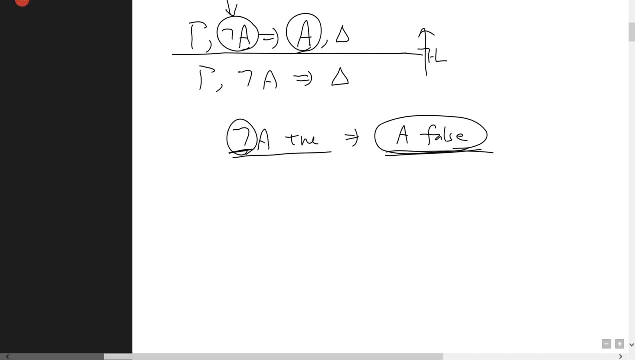 this negation A, because now we have A false as an assumption, But for consistency we keep this formula on the left side. So this is going to be negation left rule. What about negation right rule? It's completely symmetric, because if we have 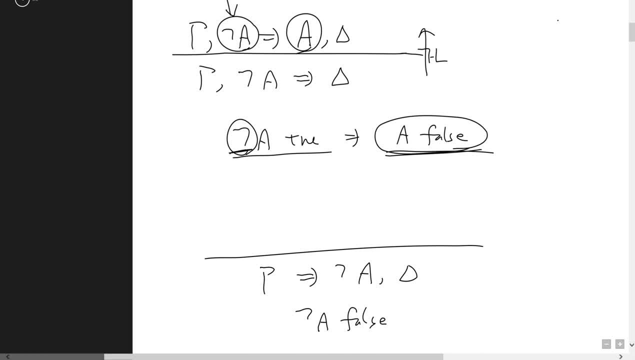 negation, A false. it means A is true, So these two statements are logically equivalent. So therefore, if we move upward, we can introduce a new assumption: A true from this one. So these two inference rules are completely symmetric. Now we have finished. 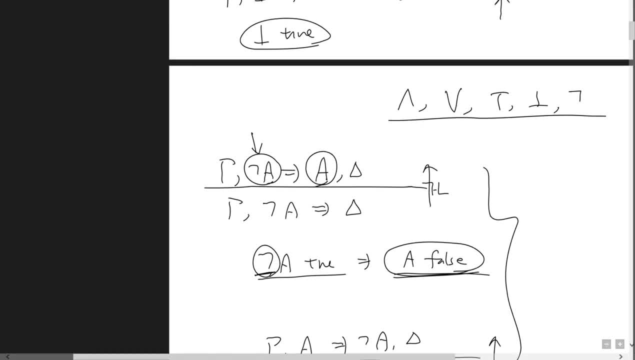 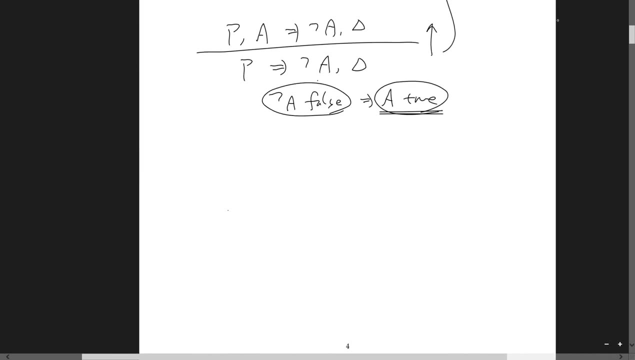 all the inference rules for these logic connectives And it remains to formulate inference rules for implication. But it turns out that in classical logic there is no notion of implication because we have this conjunction, this assumption, top and bottom and negation. 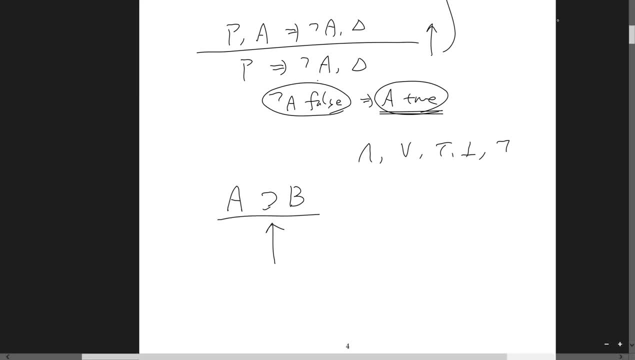 And this A implies B is actually true. It's defined as negation A- dissection B. So there is no notion of logical implication in classical logic. It's just defined as negation A- dissection B, partially because we have this law of excluded middle. 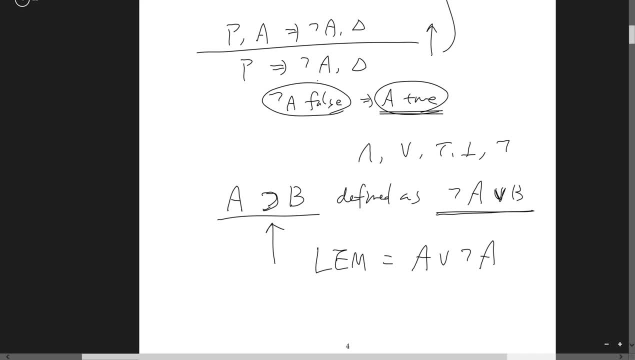 A or negation A. So for every formula we have A dissection negation A. So if we have negation A, it's a negation A. If we have A, this thing means we have B, So this thing means: 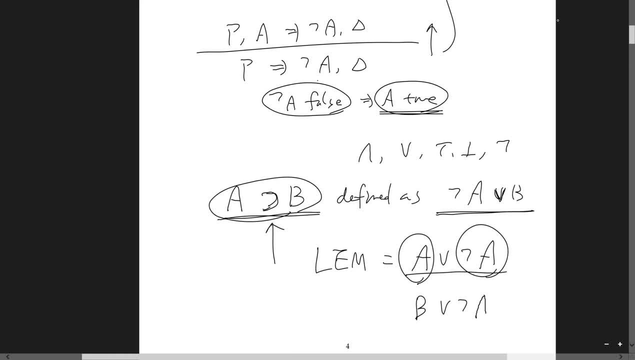 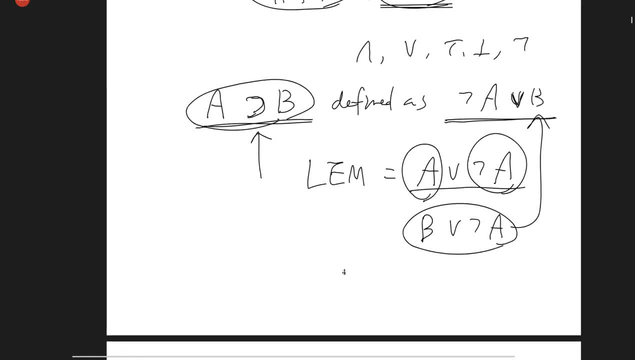 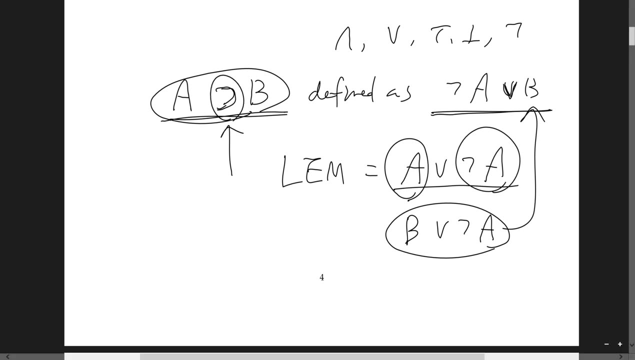 basically, we have B dissection negation A or negation A dissection B. So the bottom line is that in the case of classical logic, we don't need this extra-logic connective implication, because this notational definition, this definition A implies B. 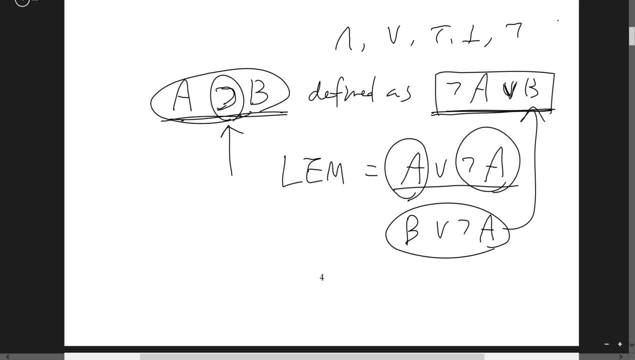 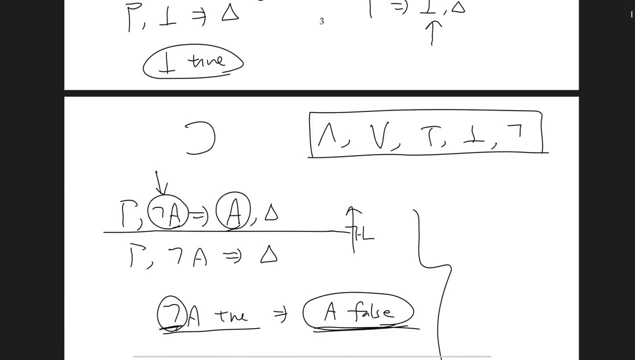 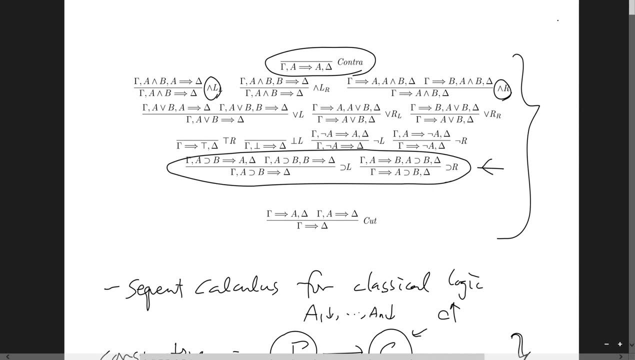 is defined as negation A, dissection B. This definition is enough. So if we go back to the system of sequence calculus, we have these two inference rules. But there is nothing interesting in these two rules because these rules are directly derived from the definition. 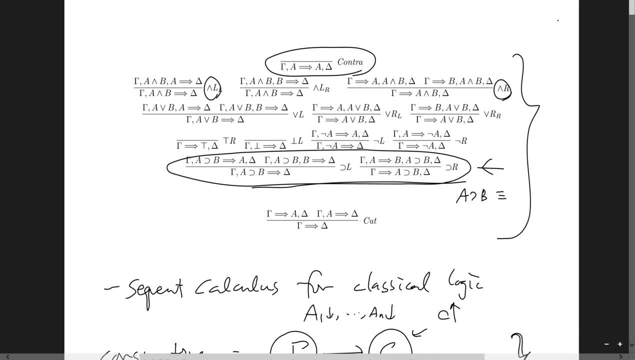 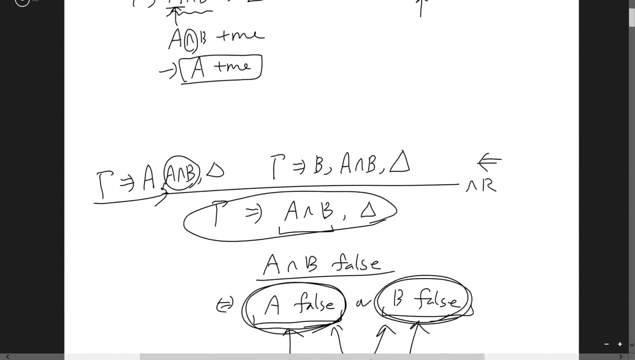 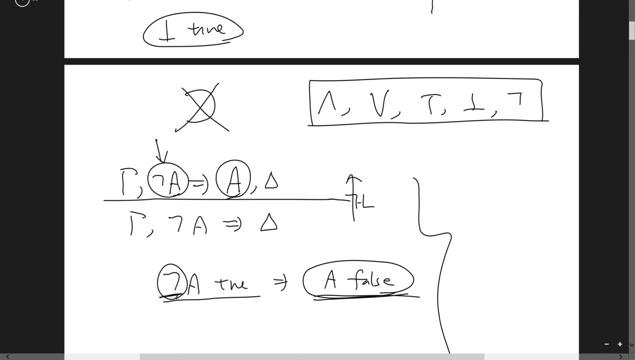 A implies B is defined as negation A or B, So we don't need this one. You can define this one in terms of negation and dissection. Perhaps the students have already learned this De Morgan's law, So we have this De Morgan's. 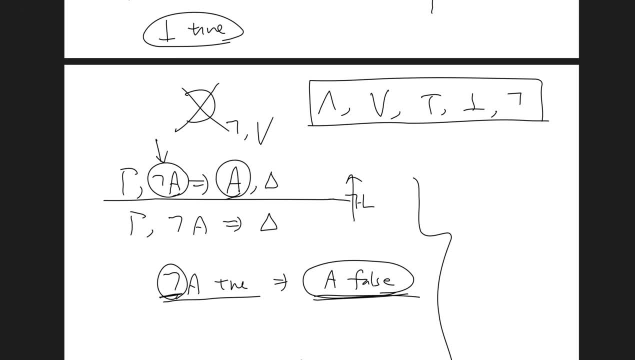 law which allows us to further simplify the presentation. So, for example, we have this De Morgan's law. for example, in the presence of a conjunction, we can define a dissection In terms of this conjunction. for example, A dissection B. 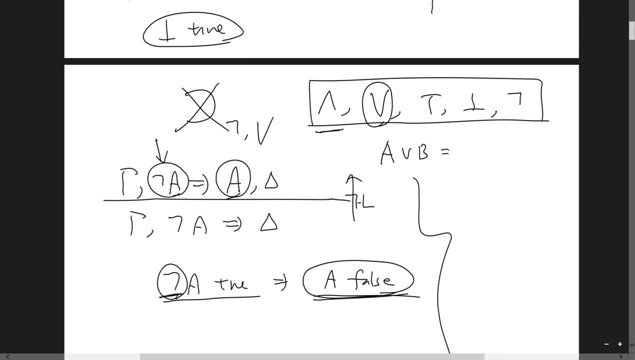 is in classical logic. well, this is logically equivalent to double negation of A dissection B, and we apply this De Morgan's law and we have negation A, conjunction negation B. So it turns out that even this dissection can be derived from. 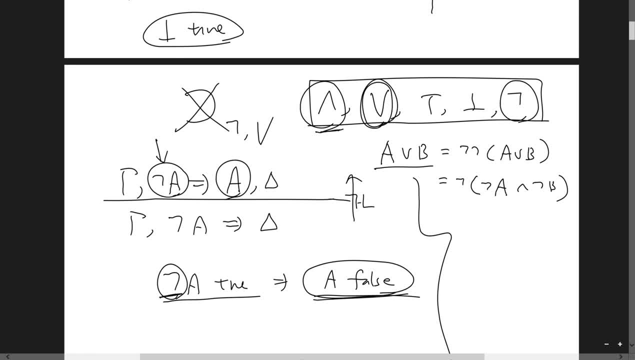 the combination of conjunction and negation and vice versa. That is, if we start with this dissection, you can actually define conjunction in terms of dissection. So we only need one of these two. If you have a top, you can define. 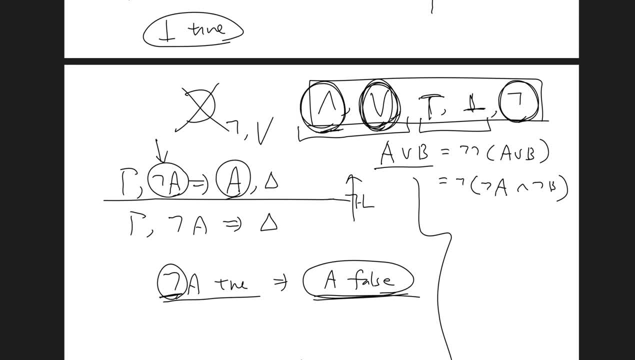 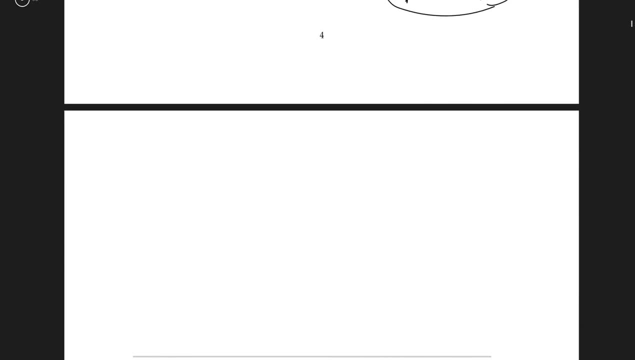 bottom as the negation of top, and vice versa. So perhaps you can get rid of this one, and perhaps you can get rid of this one, and that's all you need. Now let's investigate the methodological properties of this first conjunction property. 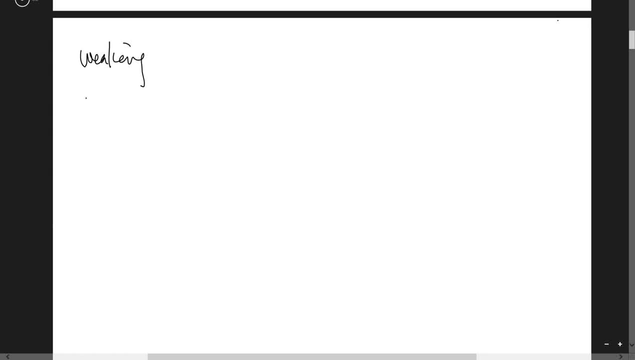 So we have weakening and contraction. So weakening is if we have gamma, double arrow delta and we can either the left side producing this one or we can contract it. This is weakening. What about contradiction If we have two copies of formula A on the left? 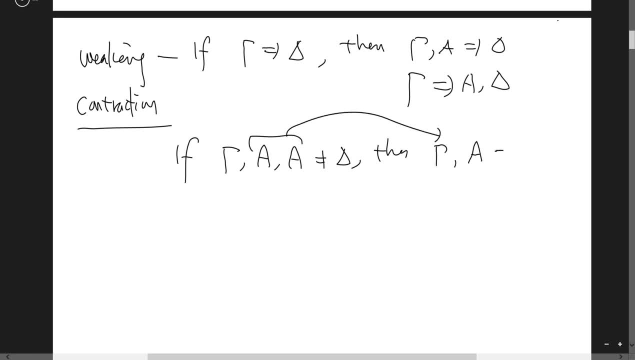 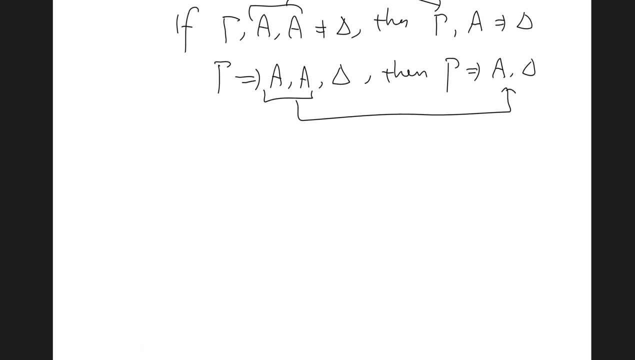 side, we can contract them into a single copy, And similarly on the right side. if we have two copies of the same formula on the left side, we can contract these two copies of the same formula. And finally, we can discuss this: 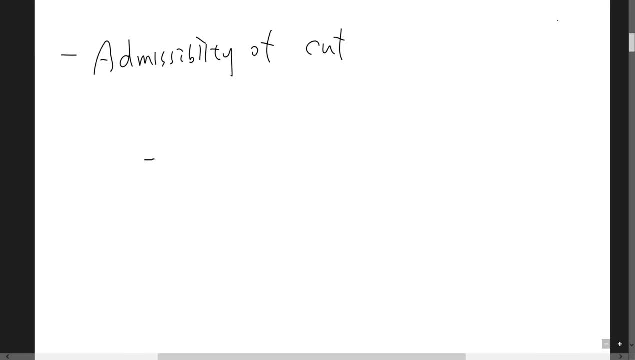 cut rule or the miscibility of cut rule. So cut rule is defined like this: If you have two copies of the same formula, then you can apply this cut rule, So you can actually apply cut, So you actually cut it away to produce. 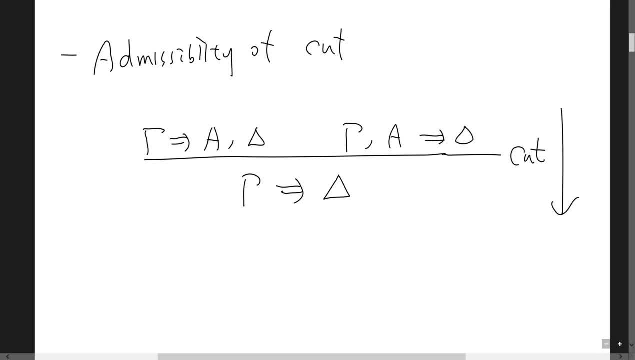 gamma double arrow delta. This is the way you generate something and then use this something as an assumption. So you just apply: cut. If you find the same formula on the right side, on the left side, then you can cut it away. So this: 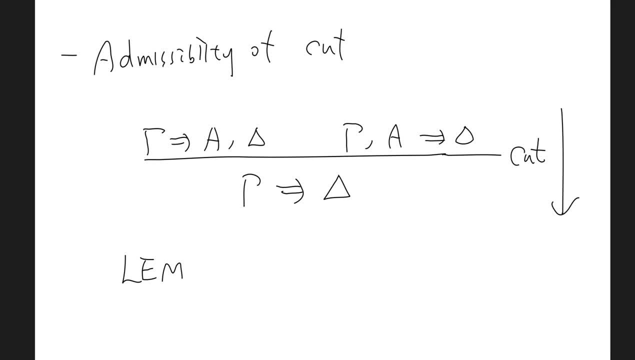 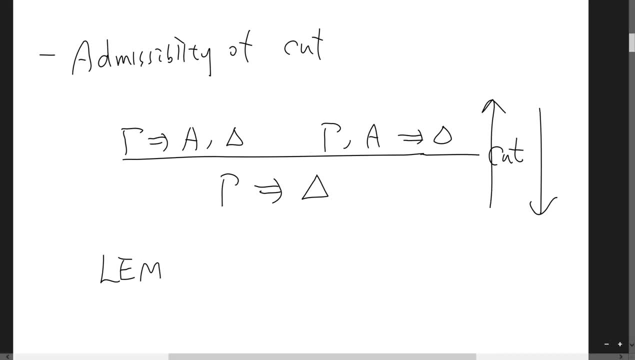 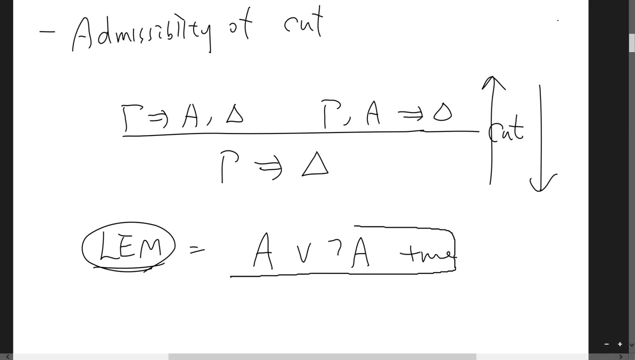 is the presentation of sequential calculus, Actually the presentation of classical logic. So, for example, if we read this rule bottom up, it precisely coincides with the interpretation of the formula. So you can add this assumption for free at any time. 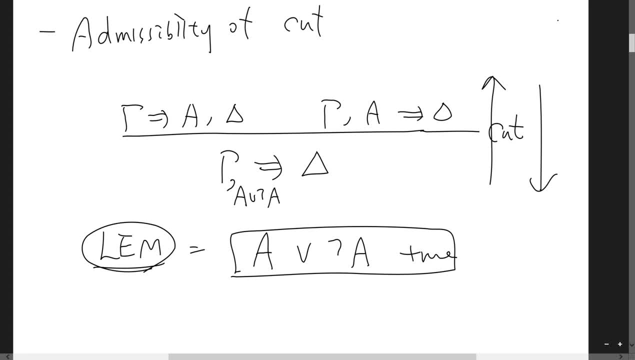 So that means that you can imagine that there is an extra assumption, a, which is invisible but it's there. So for this assumption, you create these two sequences And when you focus on this negation a, actually the formula a is moved from negation. 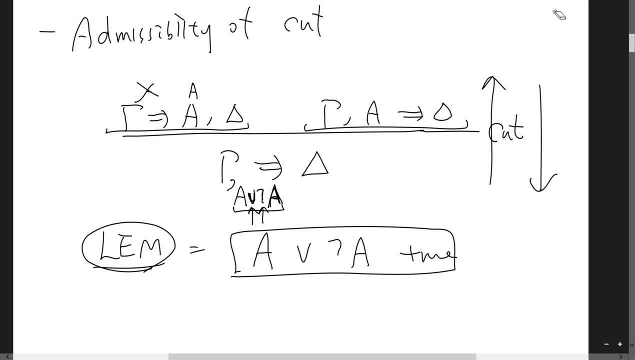 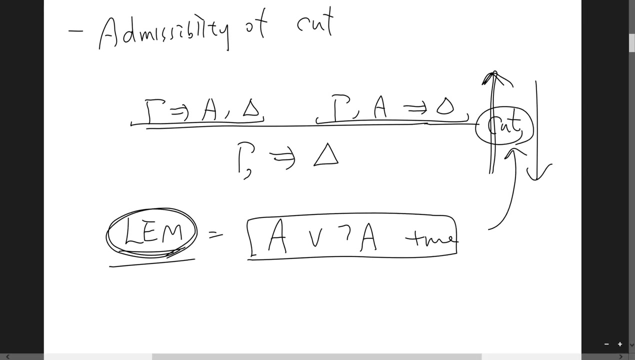 a is eliminated and we generate a new formula. So if we read this rule bottom up, we realize that it's just an application of using low over excluded middle. In this regard, we can say that this cut rule is admissible And the 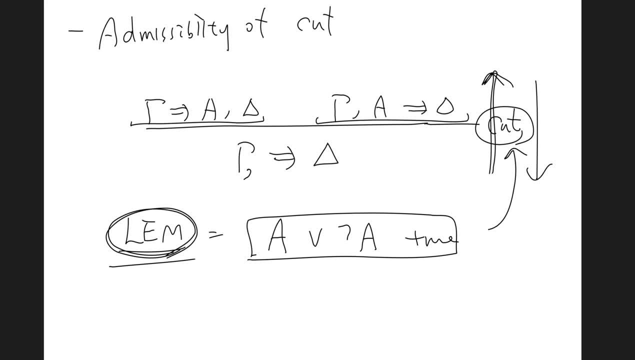 proof is actually simpler than in constructive logic.